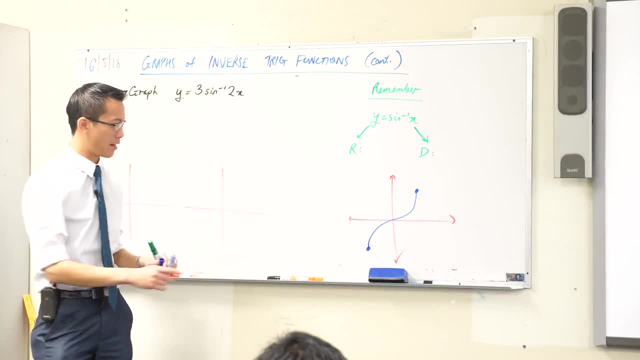 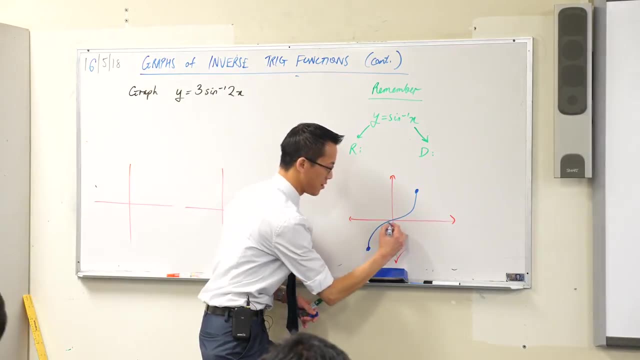 like a tangent. okay, Some of the graphs that I've seen around, you're starting to get a little bit, a little flimsy over there. it looks like you're not gonna have a tangent there. please be watchful for it. okay, Now we've got zero here. how do you remember that sine inverse is the? 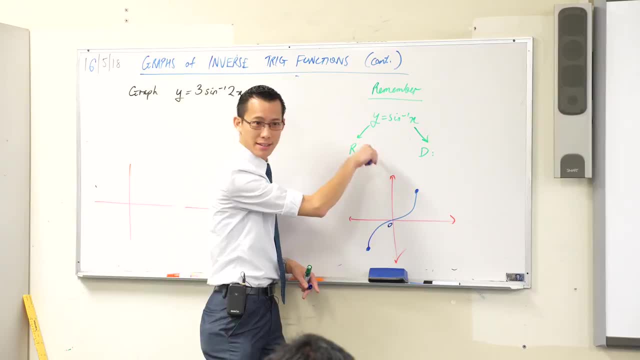 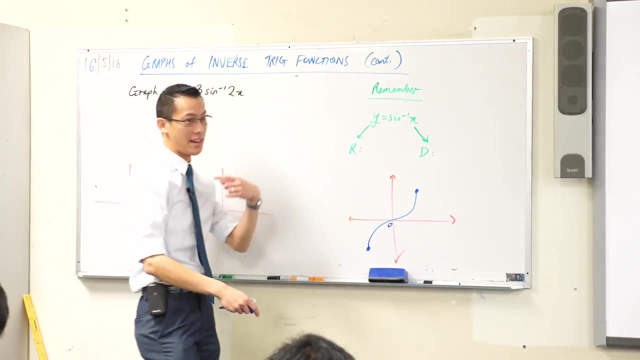 one that goes up and cos inverse is the one that goes down. There's lots of ways to remember this. I mean, you just draw lots and lots of them and hopefully that will get it into your head, but you draw sine inverse. and then the next second. 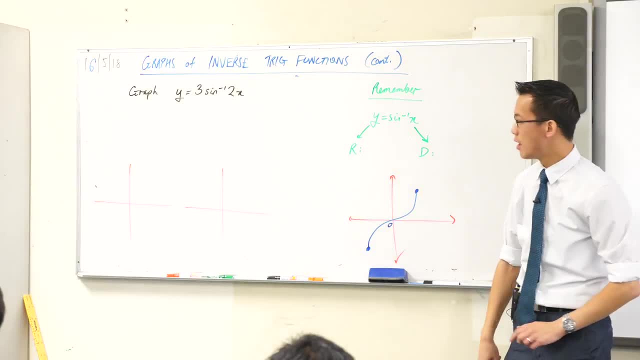 you draw cos inverse and, if you're like me, I got very confused between the two of them. So I want you to. I want to remind you of something which you may or may not have looked at earlier, which is before you looked at inverse trig. 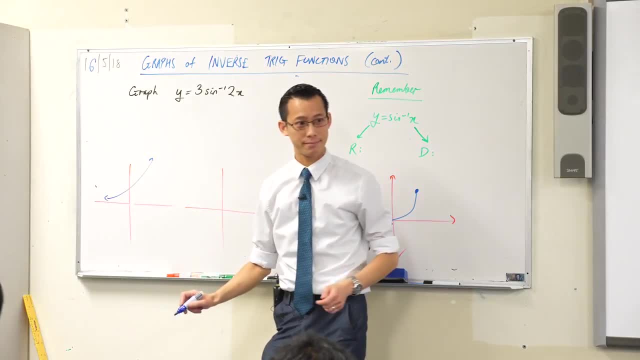 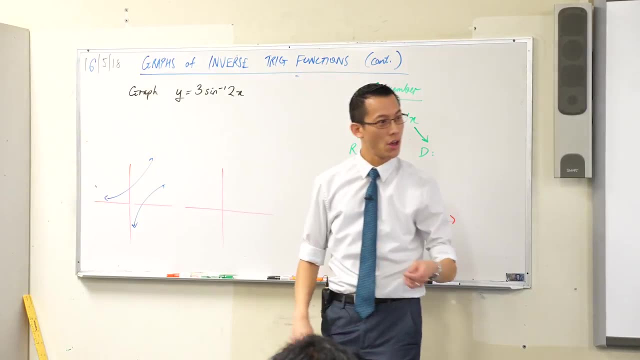 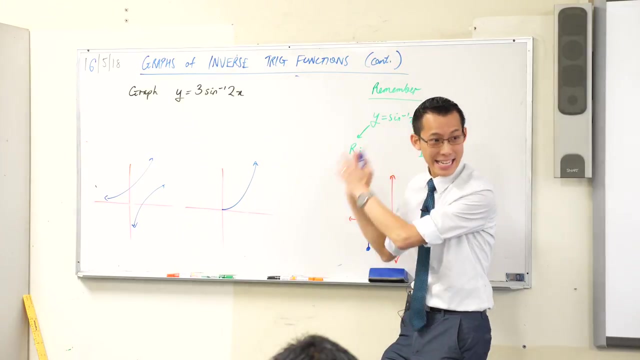 functions right. Say, for example, e to the x and its inverse, which is its inverse, which is log x right, Like so. Or we thought about functions like, say, this part of x squared, that restricted domain, and its inverse, which is the square root. 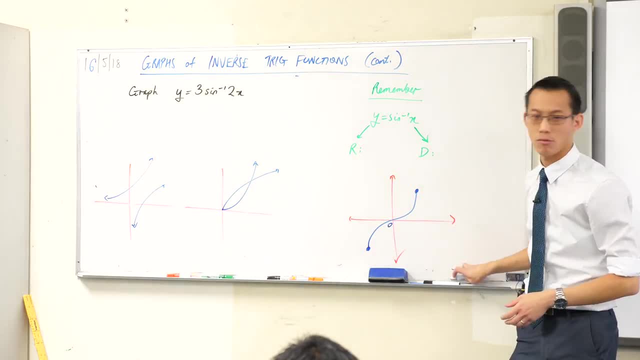 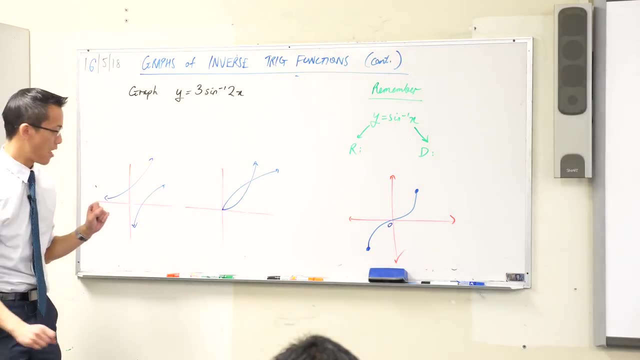 of x. okay, Now I want to call back some of the language that we developed way back at the beginning of calculus. okay, Both of these functions are what we call. throw some language at you, okay, We? these are both monotonically increasing okay. 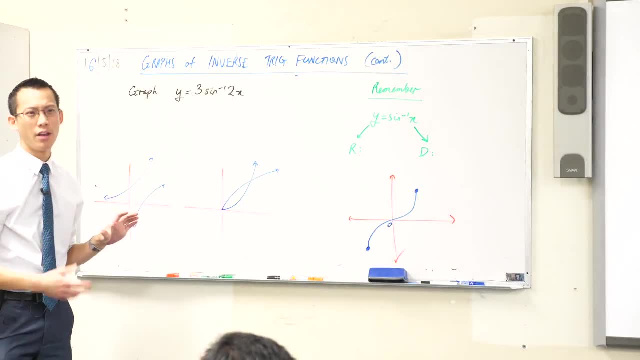 What that means is what happens when someone is monotone. It means they are talking in the same way all the time. their voice never goes up, it never goes down. that's what monotone means, right? Monotonically increasing means it's. 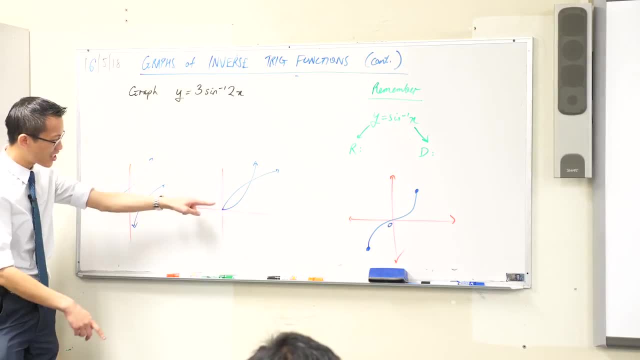 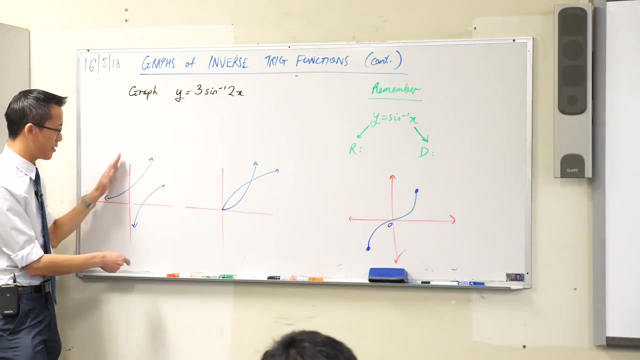 always going up, even if the x never turns around. x, squared in this domain, never turns around, okay, So it's always going up. Can you see what that means? if you look at the original function, the original function, what does that mean about its? 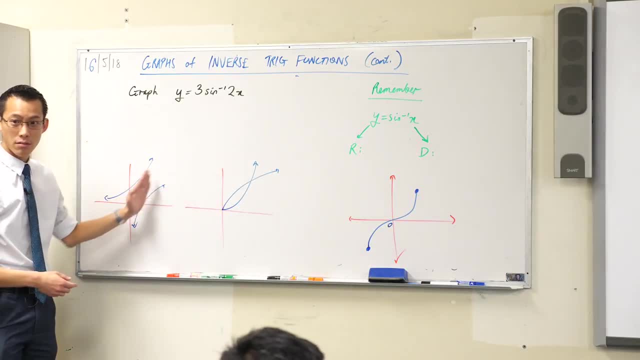 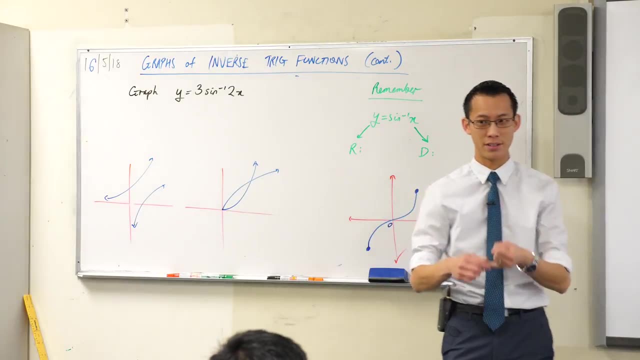 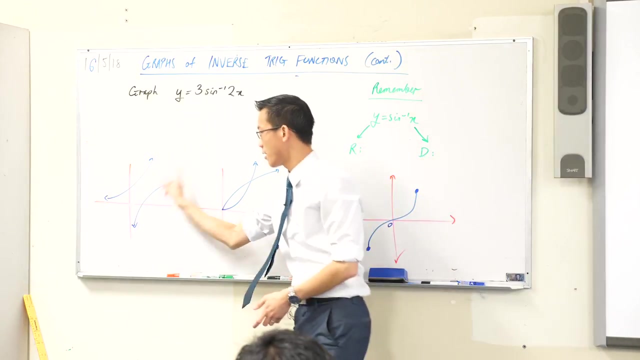 inverse. well, look at log X, look at the square root of X. do you see that if your original function is increasing monotonically, then your inverse is also increasing? do you see that? you see how, yep, I'm going up, I'm slowing down, but I'm still going up. and this guy's also going up. okay, which part of sine? because 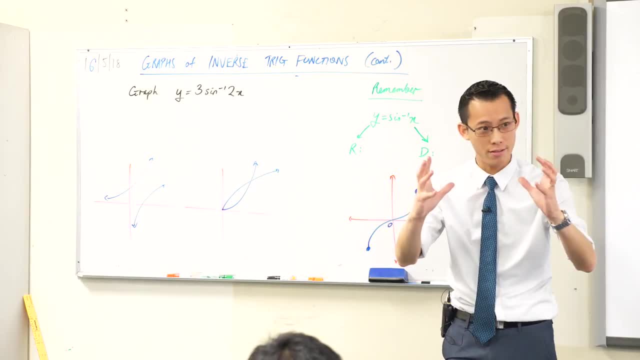 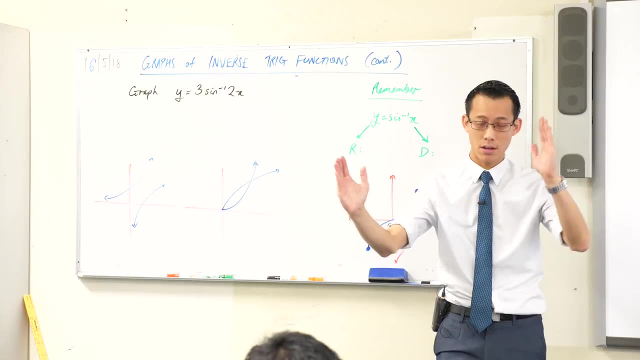 we don't do the whole thing. which part of sine do we convert into the inverse? what's the domain? it's from negative pi on 2 to pi on 2. think about what the sine graph is doing. I'm just going to hijack this. think about what the sine. 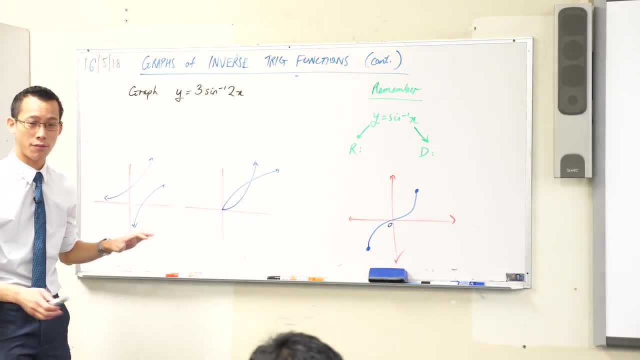 graph is doing in that particular domain, from negative pi on 2 to pi on 2. it's um, it's increasing, isn't it? and so it stands to reason that its inverse will also be increasing. make sense, and the reverse is also true. what about cos? which part of the domain? 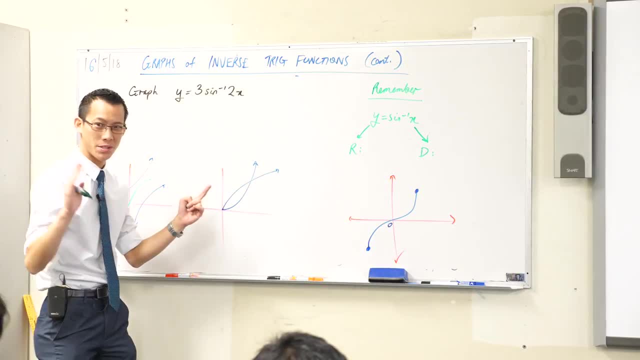 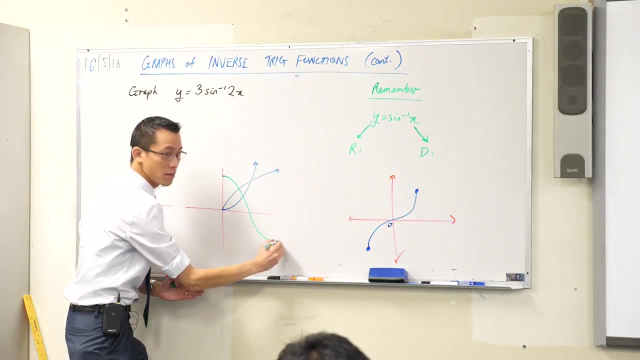 do we take to turn into cos inverse? where do we start? we start at 0 and then we go all the way to pi and in that domain cos is decreasing. you see that it's gone down, which is why its inverse is not that guy, its inverse is 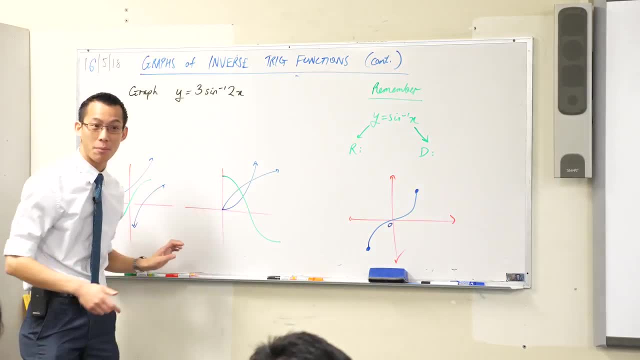 decreasing. is that okay? all right, now I need you to help me with the numbers here. you can use the graph to help you. right, and we already sort of answered this question, so I'm going to show you how to solve this problem. so I'm going to. 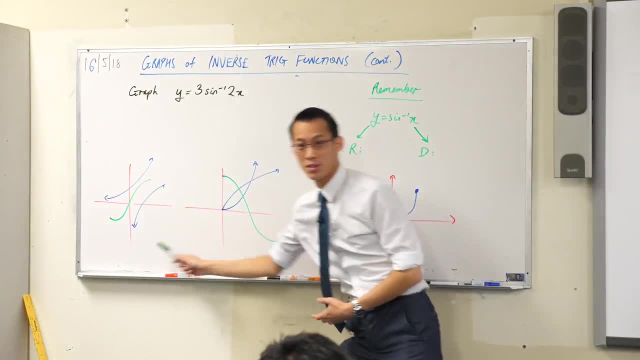 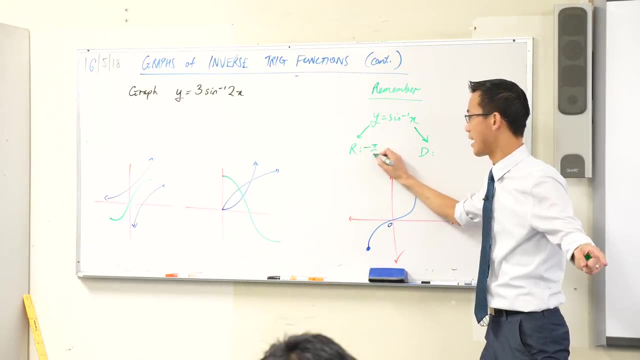 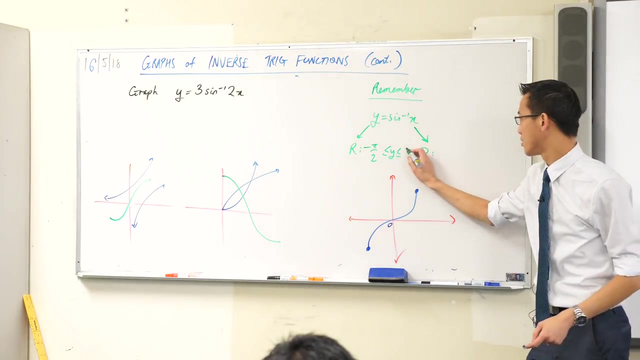 answer this question. what is the wrong color? what is the range of this sine inverse graph? how low, how high? negative pi on 2. do I include the boundary? yes, I do. that's why I have filled circles, why? and then it goes all the way up to pi on 2- fantastic, what. 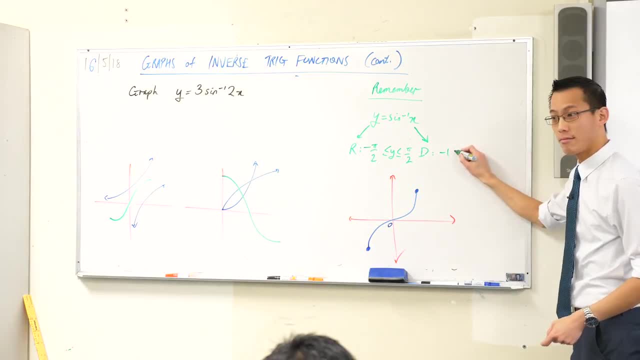 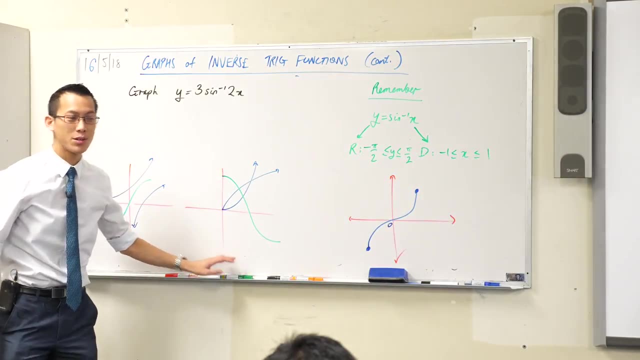 about the domain. this is even easier. negative 1 all the way to 1. are you okay with that? right now, we need to get those facts imprinted onto our brains because they will then help us when we get to this. okay, If this is what we want to graph and 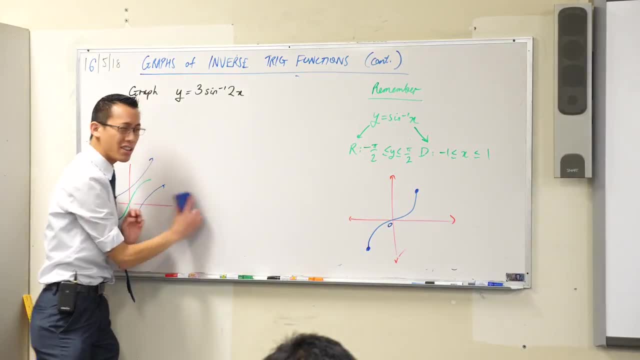 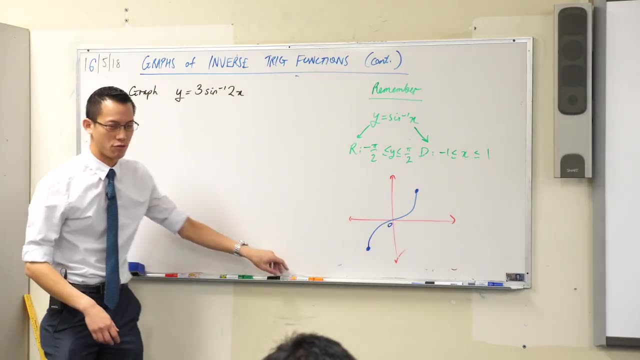 not just the regular version. okay, what we're going to do is, algebraically, we're just going to shuffle things around so that we can see the range and the domain. This might seem a little backwards to you, but I promise it will make sense by the end why I do it this. 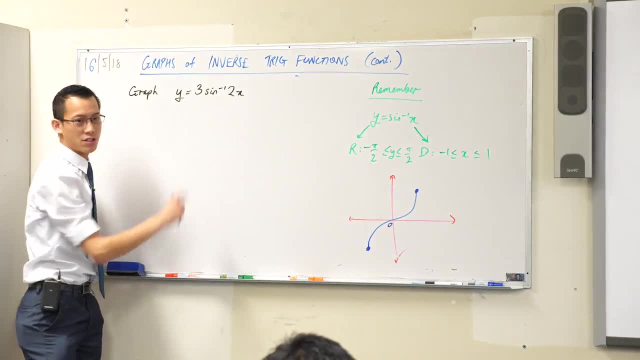 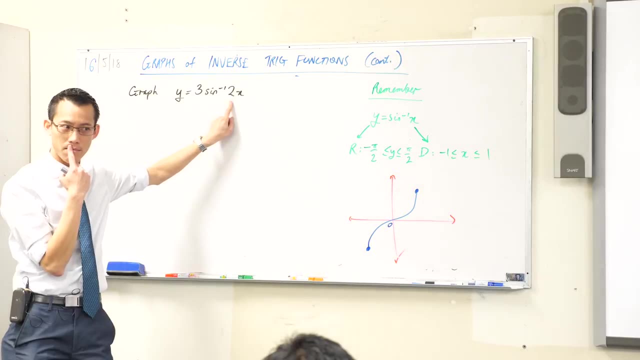 way. okay, Firstly see this 3 and this 2, right, I'll start with the 2 first. Does this alter the shape? horizontally or vertically? It's a stretch or a scale? Which way is it? It's horizontal. How can you tell that it's horizontal? It's attached to the x which. 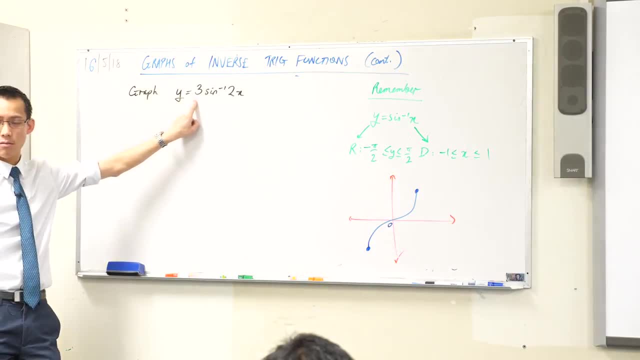 is the horizontal axis. yes, What about the 3?? That changes the range. it changes it vertically. To make that a little bit clearer, I'm going to put the 3 where it really belongs, which is with the vertical variable. is that okay? So I'm going to write it like this: 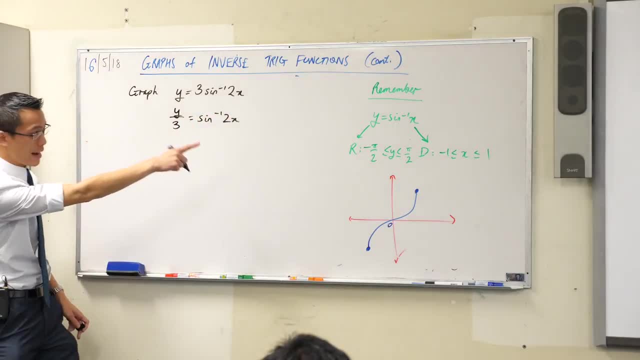 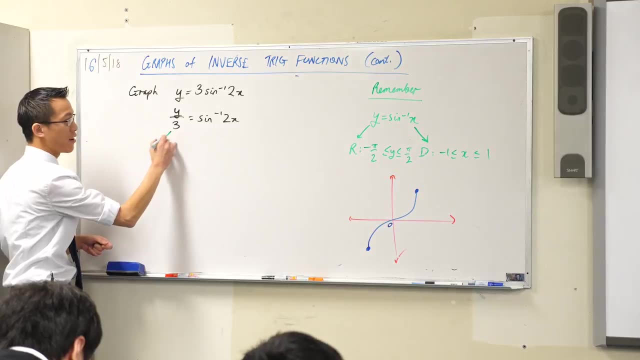 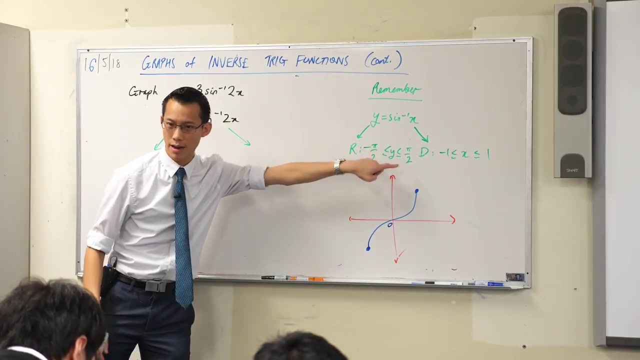 Is that okay? Now you see how I got range and domain out of the y and the x. Well, this is sine inverse, just like that is. so I can get the range and the domain out of these guys, right. But the difference is I don't have y between negative pi on 2 and pi on. 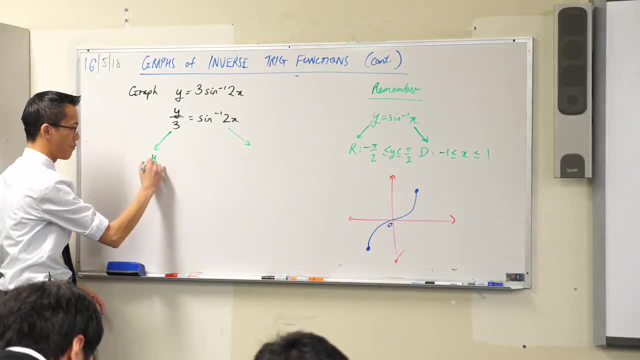 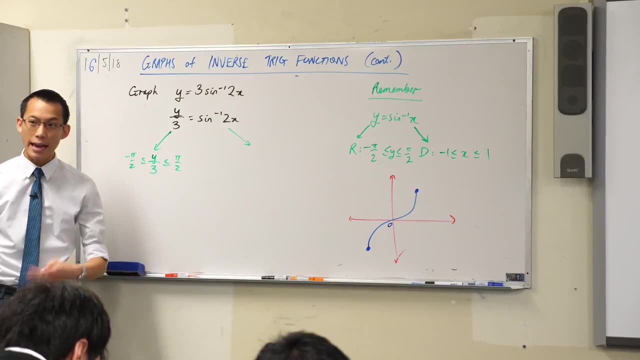 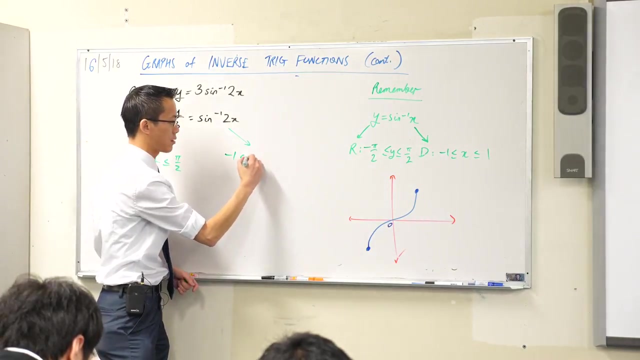 2.. I've got y on 3, that's what exists between negative pi on 2 and pi on 2, okay. And in the same way, I don't have x between negative 1 and 1. I've got 2x. so that's what I'm going to write like. 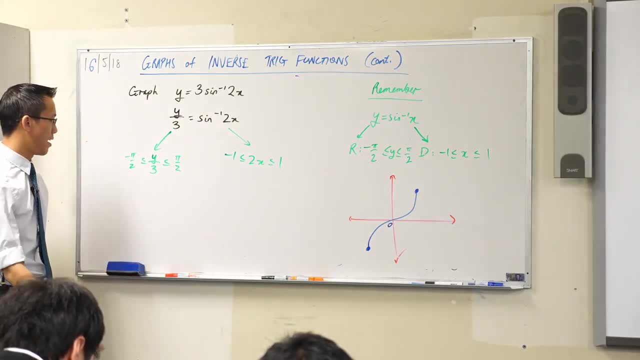 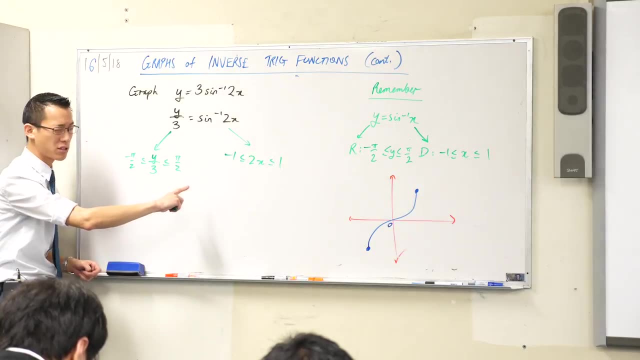 so okay. so the real range and the real domain are simply y and x on their own. so you can see, in this case, all I have to do to the whole inequality. what do I do? I'm just going to multiply by 3 and that gives you negative 3. pi on 2 all. 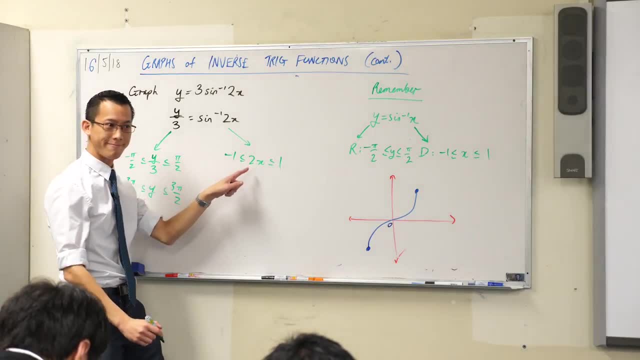 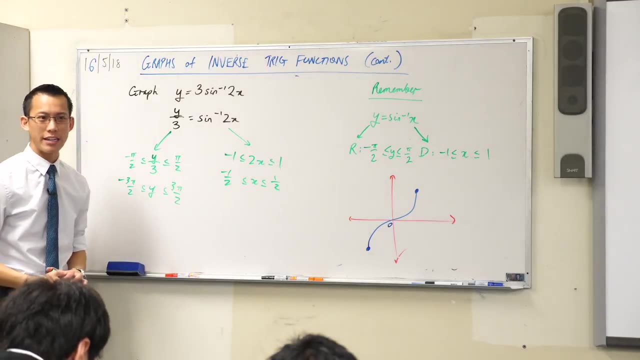 the way to 3. pi on 2. what about this one? what will I do? divide by 2 bingo. okay, now many of you are going to say: I already knew that. that's what it was going to be. I can draw this now. in fact, I'm going to hijack this graph over here. 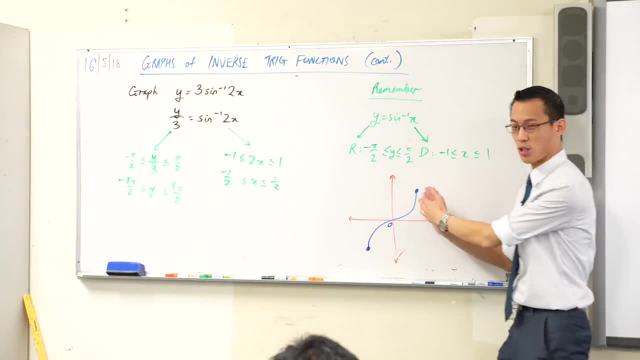 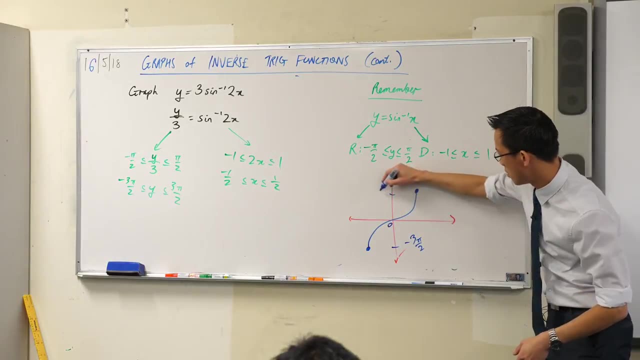 that's how cheap I am and I'm going to say it's exactly the same, except it just won't go as far, right, or we'll go further. so range is from negative 3 pi on 2 to 3 pi on 2. the shape is preserved. and from here to here, what are those? 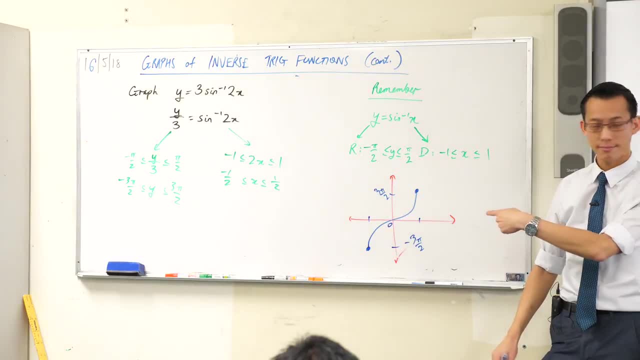 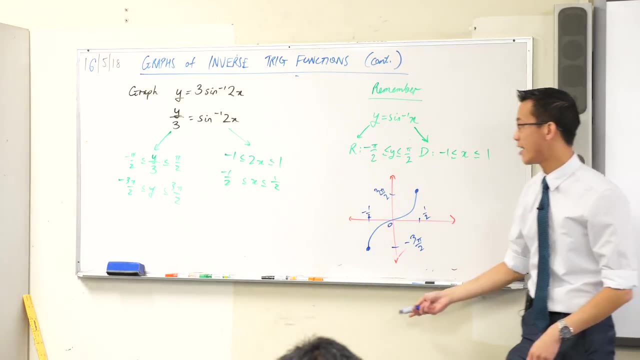 boundaries going to be. what does the domain tell me? you, negative, a half to a half. okay, and you're done. now many of you will say I could have drawn that without thinking about the domain and range in this strange way. let me give you two reasons why I'm going to encourage you to do.